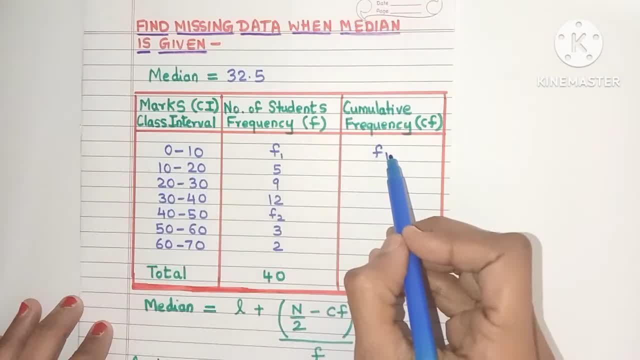 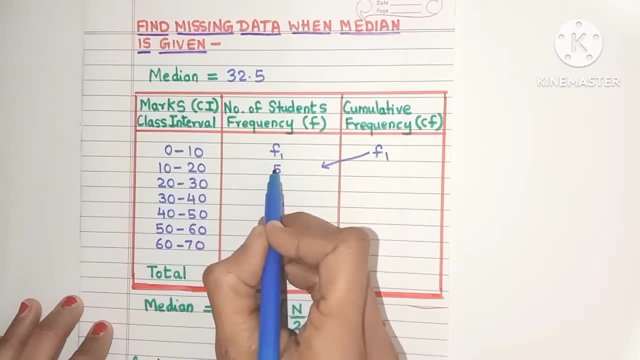 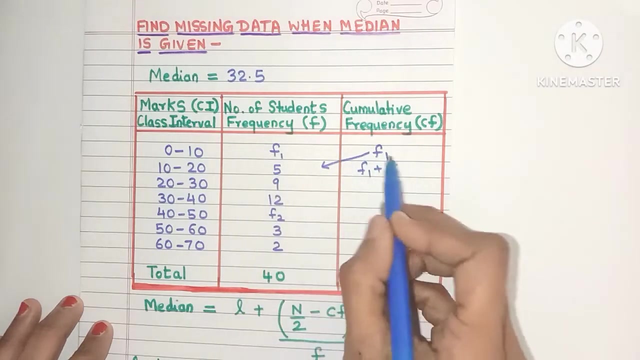 class interval. So this is my previous class interval, and its cf value is f1.. So you simply add f1 to the frequency of the present class interval, which is nothing but 5.. So f1 plus 5.. Now, because f1 is a variable and 5 is a constant, you just have to leave it like this, friends. So 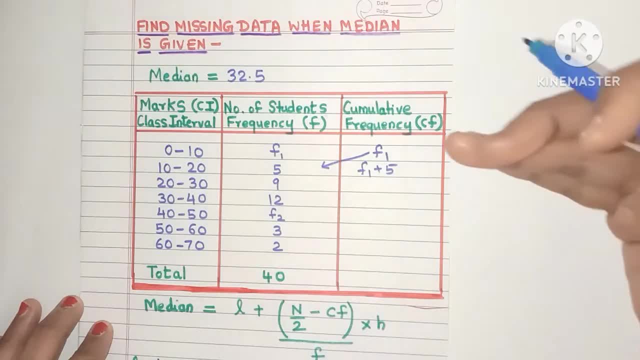 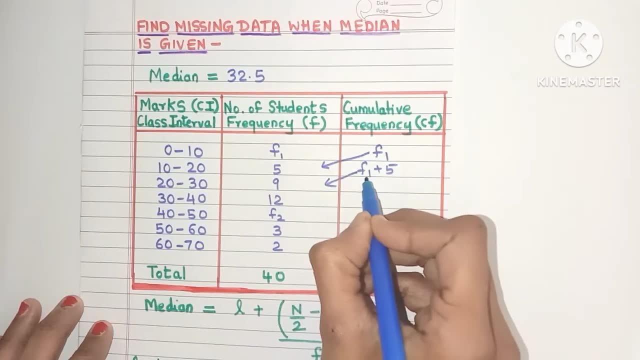 it will be f1 plus 5.. I hope you understood this, friends. Now you need to simply repeat this process for all the class intervals. So let's do that. So here for the next class interval, I will get the cf value as f1 plus 5 plus 9.. So 5 plus 9, you can definitely add, because they both 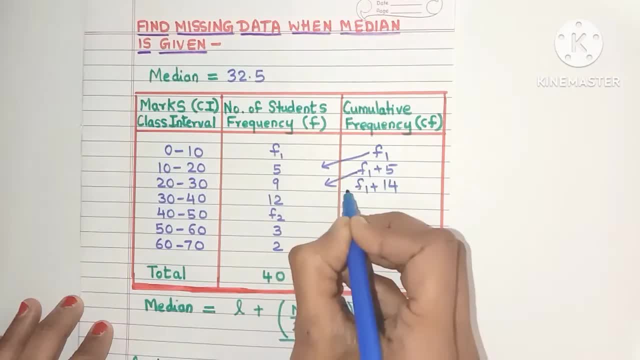 are constants, So we will get f1 plus 14.. Now for the next class interval. we will get f1 plus 14 plus 12 is 26.. Now here we get f1 plus 26 plus f2,, friends, Because f1 and f2 are two different. 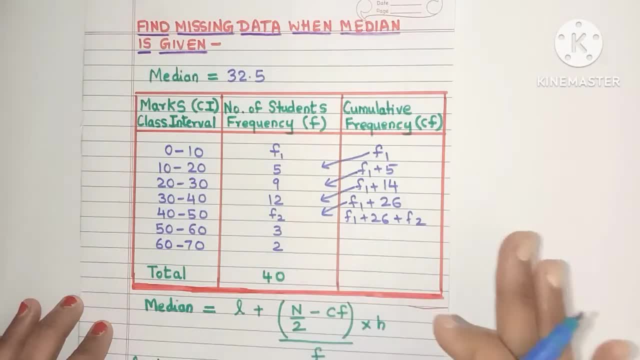 variables. we really can add f1 to the frequency of the previous class interval, So we will get f1 plus f2 plus 29. And again, when we add, we will get f1 plus f2 plus 31. And that is how we. 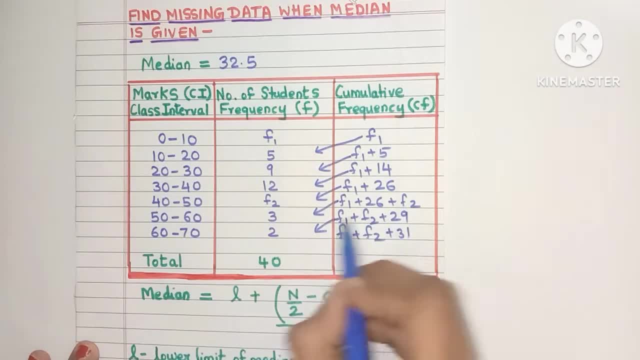 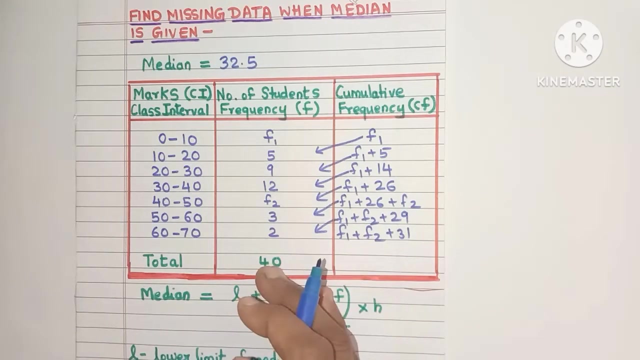 get all the cf entries Now. the last cf value always gives us the total number of observations. But it is already given to us that 40 is the total number of observations. So can we say that f1 plus f2 plus 31 is equal to 40?? Definitely, because they both give you the total number of observations. 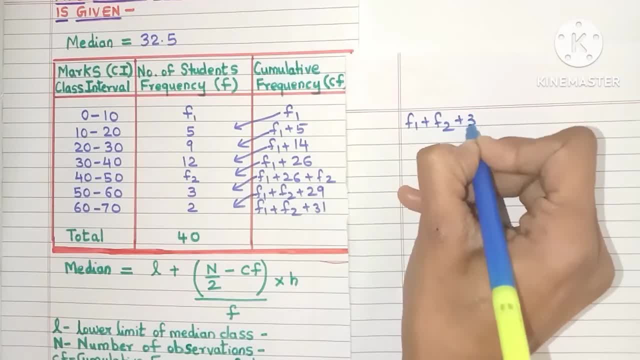 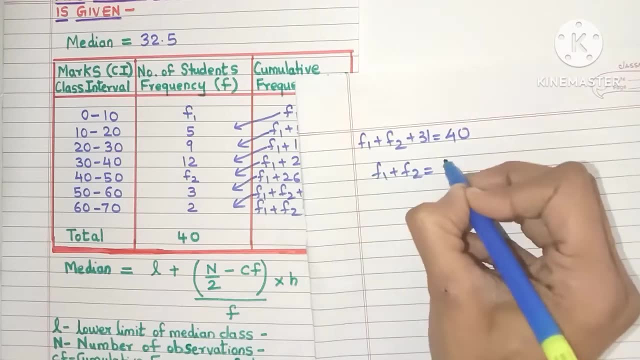 So let's write: f1 plus f2 plus 31 is equal to 40. Now you can always bring 31 to the other side, So let's do that. We will get f1 plus f2 equal to 9.. Friends, let's call this as equation number. 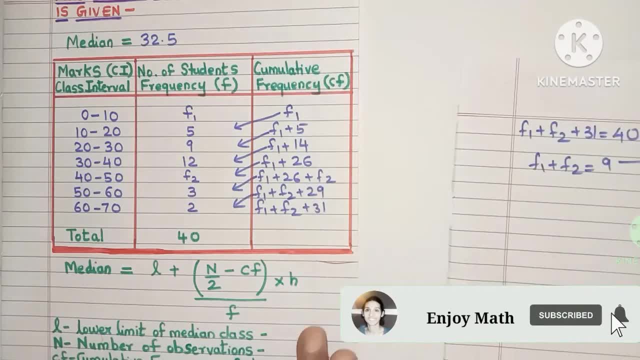 1, because we will definitely need it later. Now let's come back to the median value. Median is 32.5.. Now, in which class is this? In which class is this? In which class is this? In which class is? 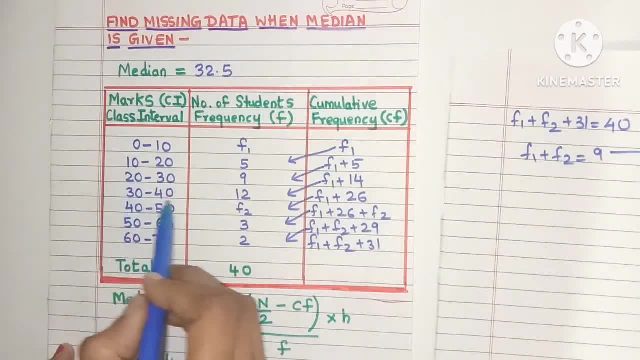 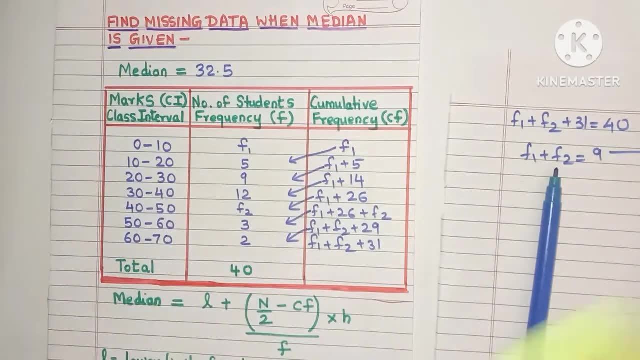 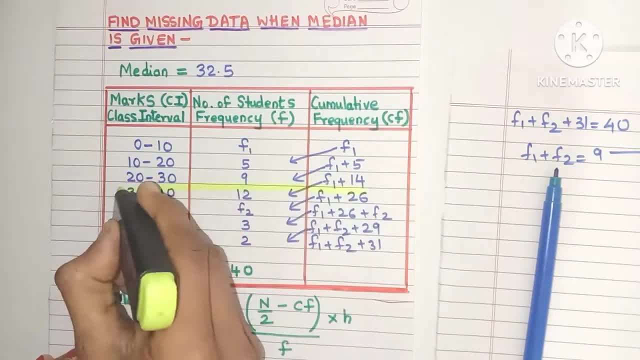 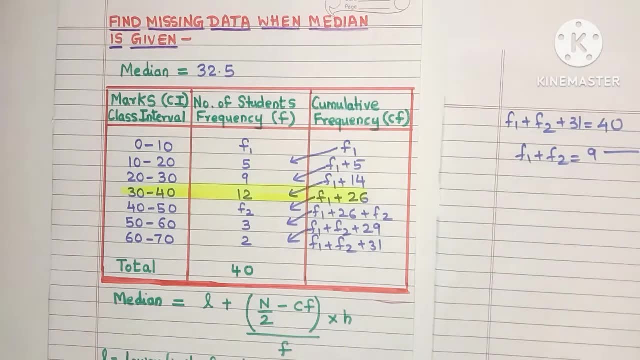 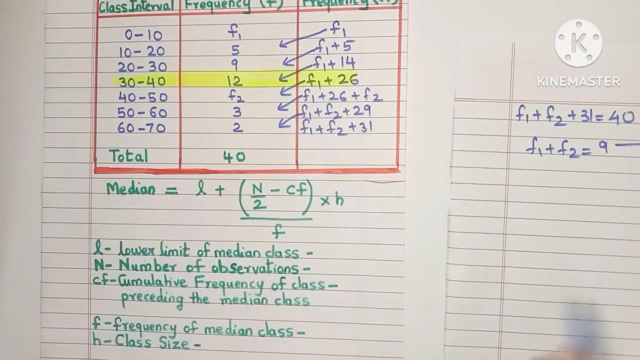 median class, friends, Let's highlight it. So finding the median class is very easy if you already know the median value. So this is our median class. Now that we know what is the median class, we can easily find out all these values. So L is nothing but the lower limit of the median. 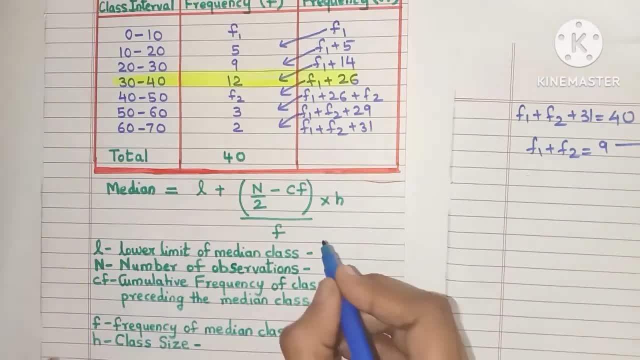 class. So this is our median class. Now let's find out the lower limit of the median class. So this is our median class. Lower limit is 30. So let's write 30.. N is the number of observation. 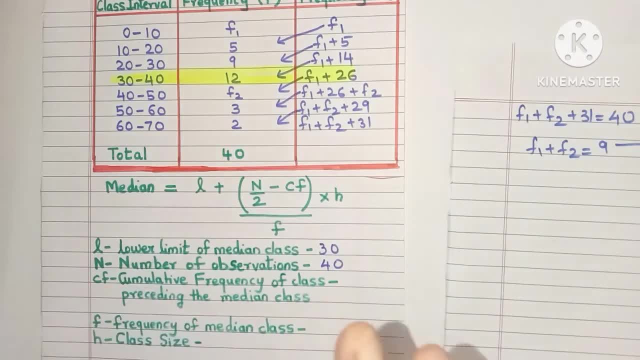 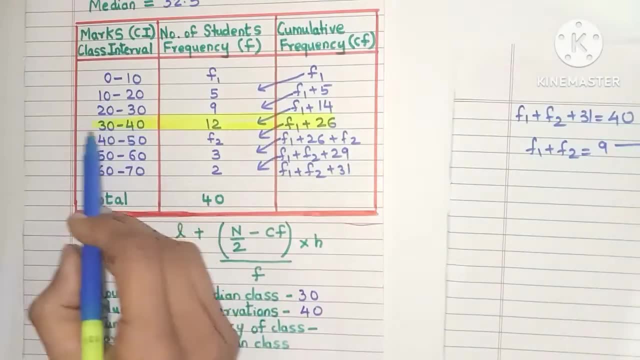 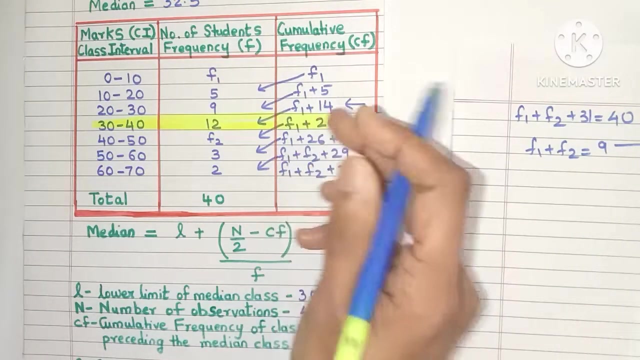 Now that's already given as 40.. CF is the cumulative frequency of the class preceding the median class. Now, preceding means coming before, So this is my median class, The class that comes before the median class. is this one, friends, And what is the CF value? F1 plus 14.. 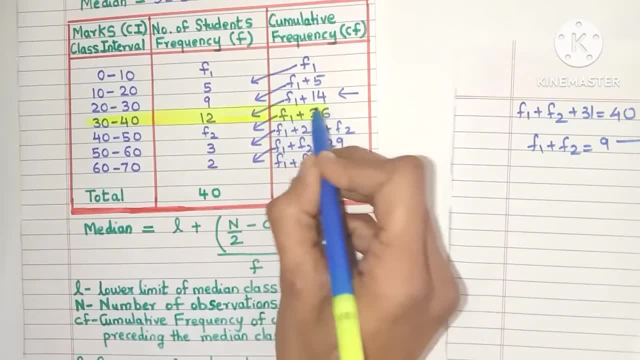 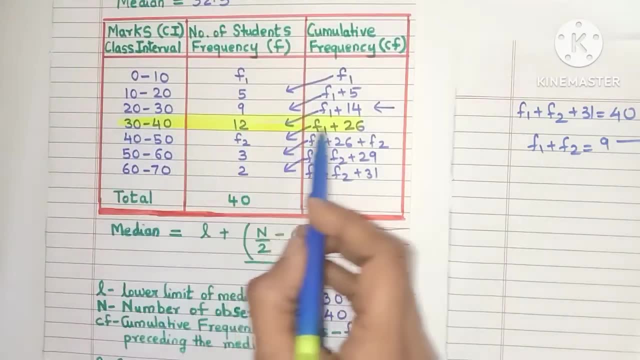 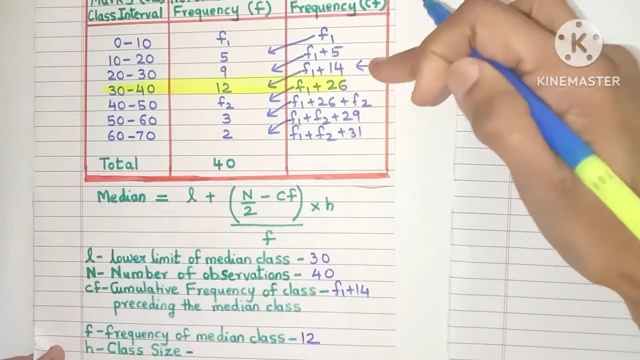 So remember not to confuse it with the CF of the median class. The next is F. F is nothing but frequency of the median class. So this is my median class. Its frequency value is 12.. So remember, friends, the CF value you have to take for the class that comes. 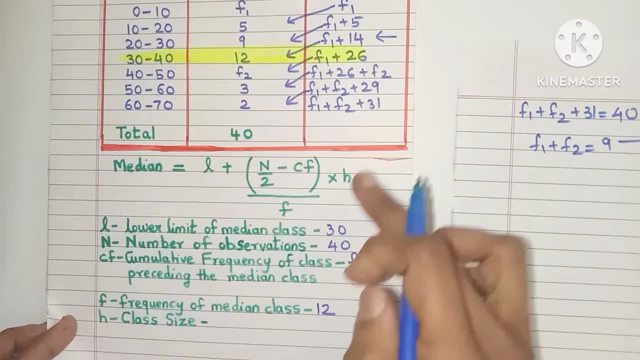 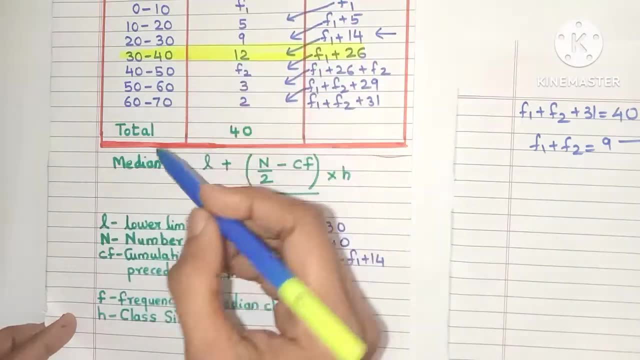 before the median class and F value you have to take for the median class. Now, H is nothing but the class size. Now that's very simple. Take any class interval, say 40 to 50, just subtract the upper limit and the lower limit, So 50 minus 40, you'll get 40. So this is our median class Now. 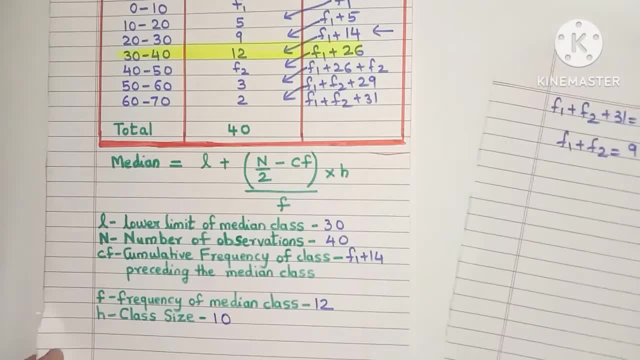 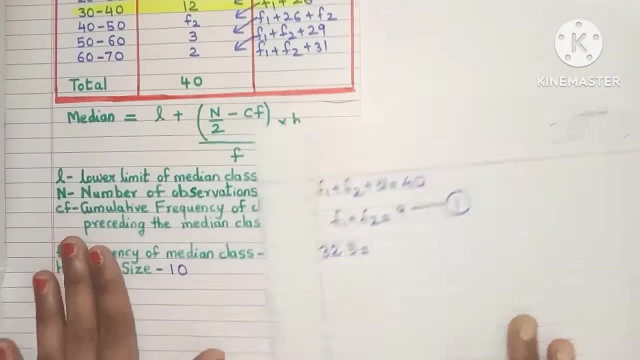 let's look at it as 10.. That's it, friends. We have got all the values. Let's substitute it in the formula for median. So median, which is nothing but 32.5, is equal to. now. what is L? 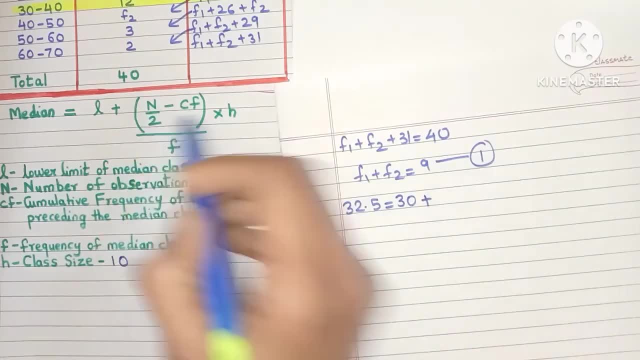 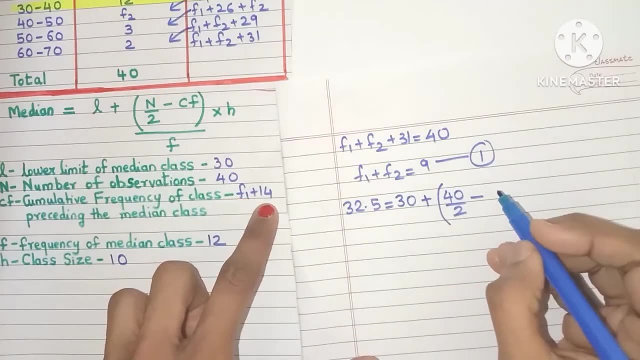 value. We just found it as 30 plus N. Let's put the bracket also. N is nothing but 40 by 2 minus CF. CF is nothing but F1 plus 14, friends. So because it's not a number, you have to write it. 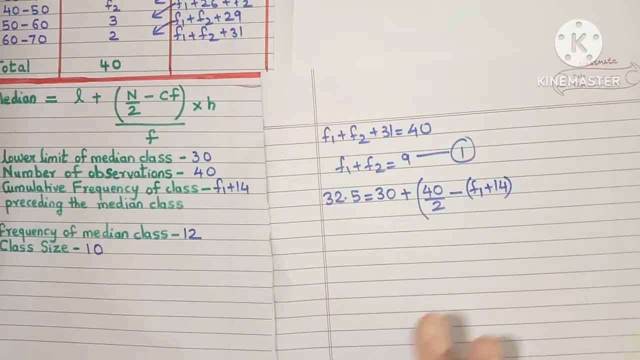 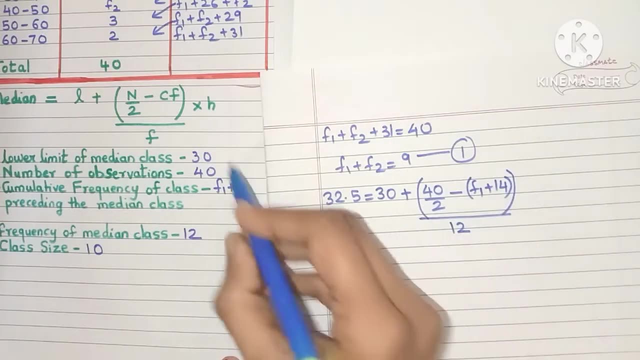 in brackets. If you don't write the brackets, your calculations will be wrong. So let's be all wrong, friends. So remember to put the brackets everywhere. divided by F, Now F value is 12, and then multiplied by H, which is nothing but 10.. Now let's continue Now. 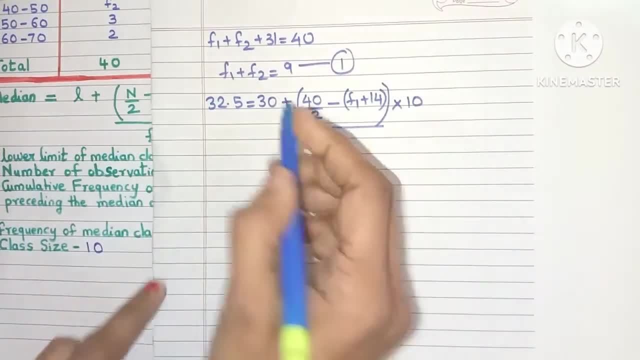 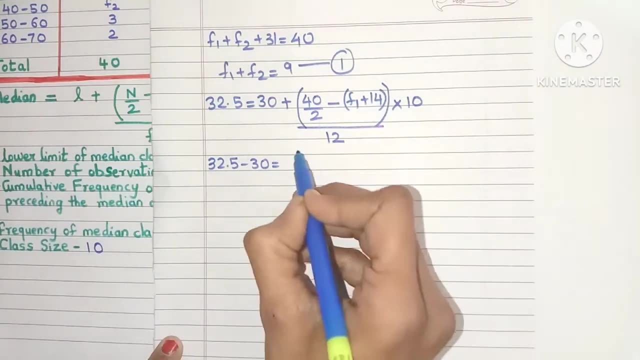 because this 30 is separate from this entire term, I can surely bring it to the other side. So here I'll get. 32.5 minus 30 equals, to let me keep the bracket. 40 by 2 is 20.. Now 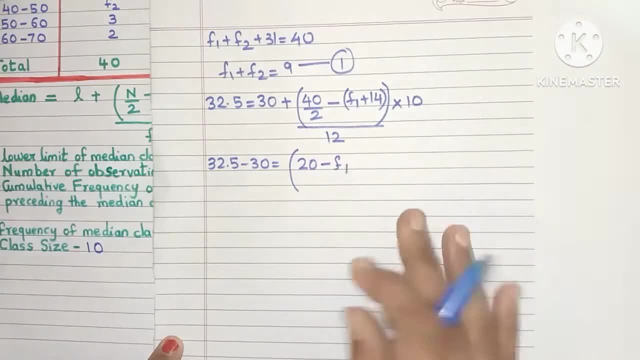 let me open up this bracket string, So I'll get minus F1,, minus F2,, minus F3,, minus F4,, minus F5,, minus F6,, minus F7,, minus F8,, minus F9,, minus F10,. 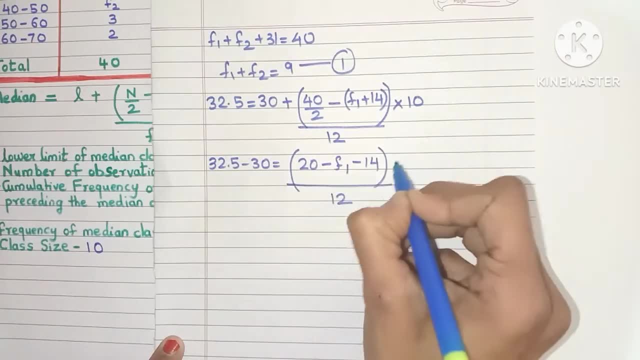 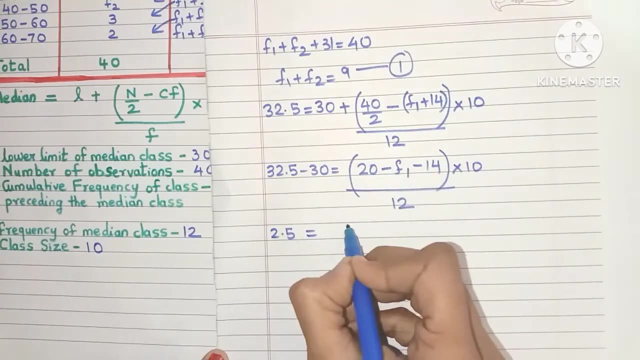 minus 14.. And let me put the bracket here, divided by 12, into 10.. Now this is nothing but 2.5 equal to Now, 20 minus 14 is nothing but 6 minus F1.. Keep the bracket as it is. 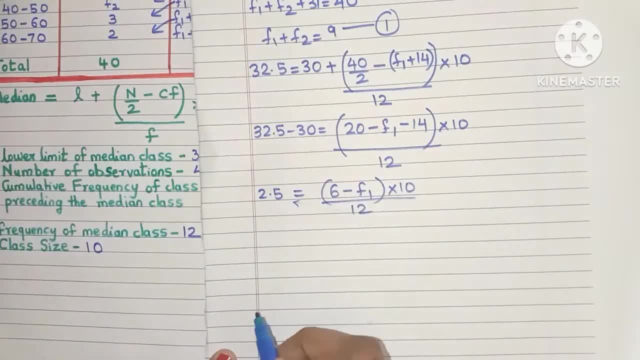 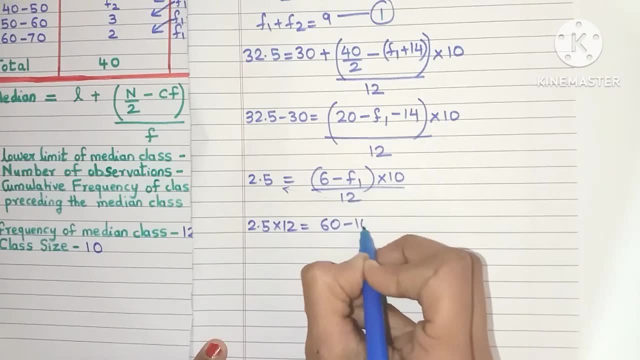 divided by 12.. Now we can always bring the 12 to the other side. friends, Let's do that. 2.5 into 12, equal to Now. let's open up the brackets So I'll get 60 minus 10 F1. Now. 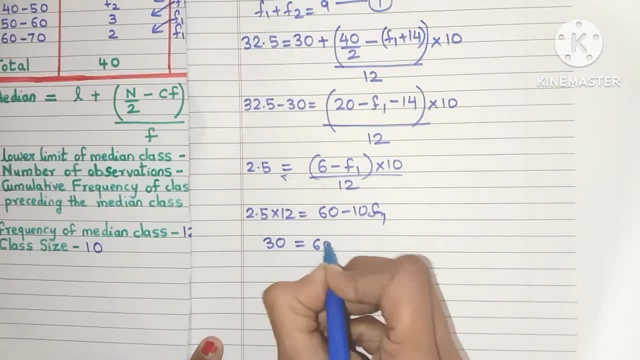 2.5 into 12 is nothing but 30. Which is equal to 60 minus 10 F1.. Now let's little bit shift the terms here and there. So I'll get 10 F1 to the other side And I'll bring 30 to this side, friends. So I'll get 60 minus 30.. 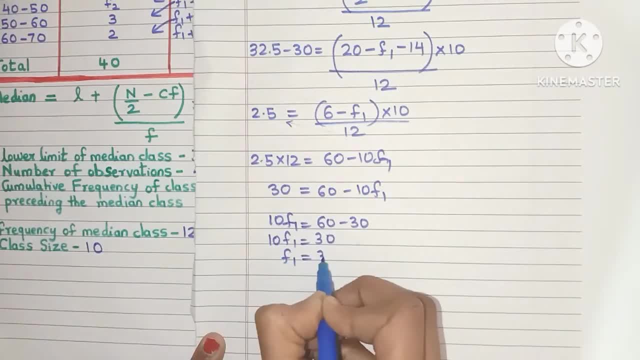 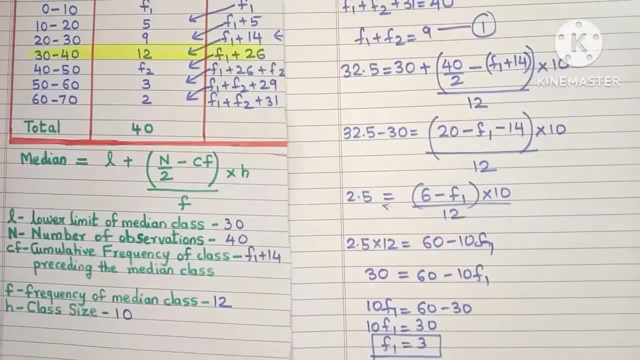 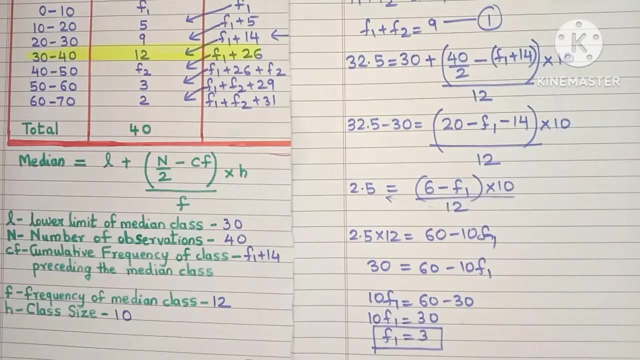 So 10 F1 is equal to 30, which means F1 is equal to 3.. So here we have easily got the first missing frequency value, F1, as 3.. Now to find the other frequency value, you simply have to substitute this F1 value in this equation number 1,. 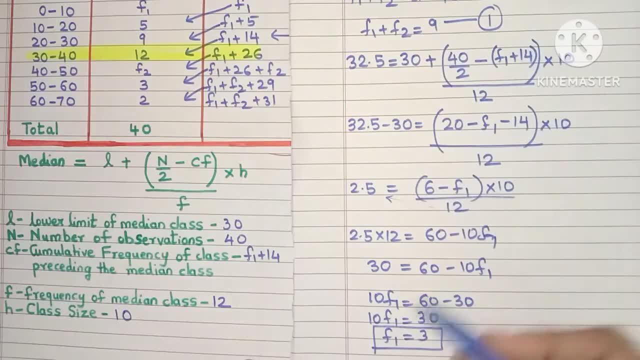 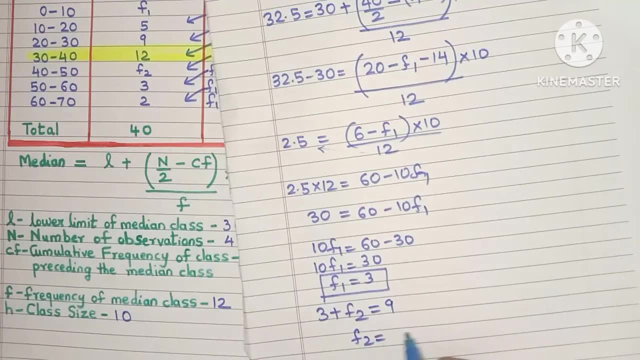 friends. So what does it say? F1 plus F2 is equal to 9.. F1 is already 3.. We just found it out. So 3 plus F2 is equal to 9. That means F2 is equal to 6.. So that's it, friends. We got the values of. 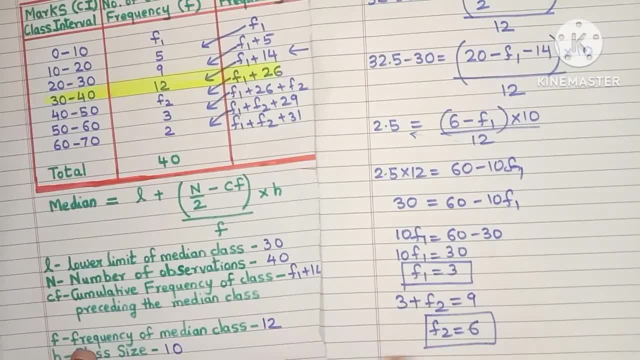 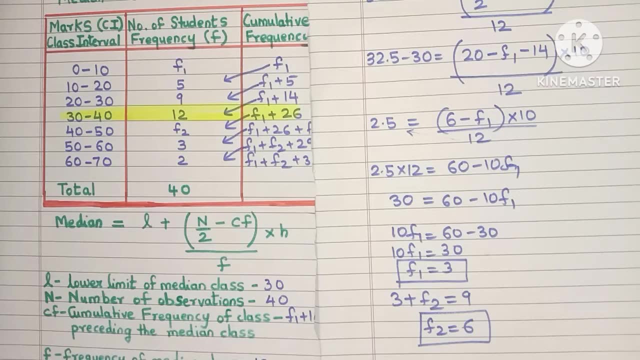 F1 and F2 very easily using the median formula. So if you found the video useful, do like and share it. Consider subscribing to Enjoy Math And please leave your comments in the comment section below. So till we meet again, take care.